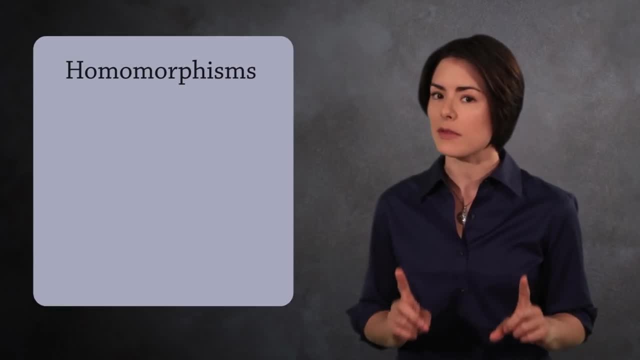 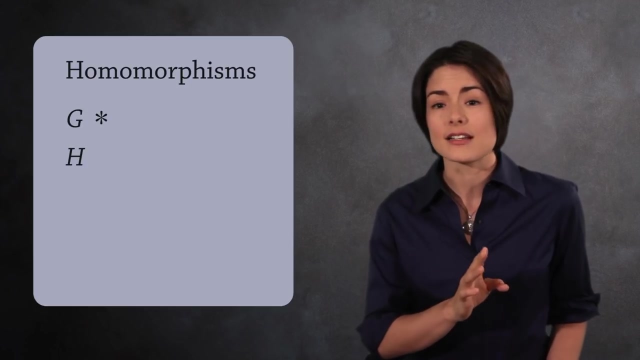 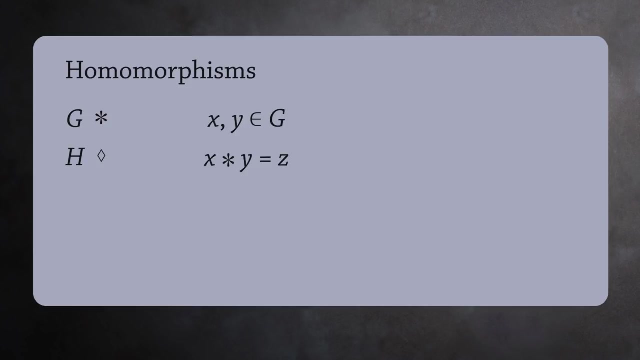 A homomorphism is a way to compare two groups for structural similarities. It's a function between two groups which preserves the group structure in each group. Let's be more specific. Suppose we have two groups G and H. Remember, G and H are different groups, and they may have entirely different group operations. To help us keep G and H separate in our minds, let's use an asterisk for the group operation in G, and a diamond for the group operation in H. We'll still use the word times, but we'll write the correct symbol for the operation. Now pick any two elements x and y in G. Let's say that x times y equals z. Next, suppose we have a function f that maps G to H. The three elements, x, y, and z are mapped to elements in H. x is mapped to f , y is mapped to f , and z is mapped to f . 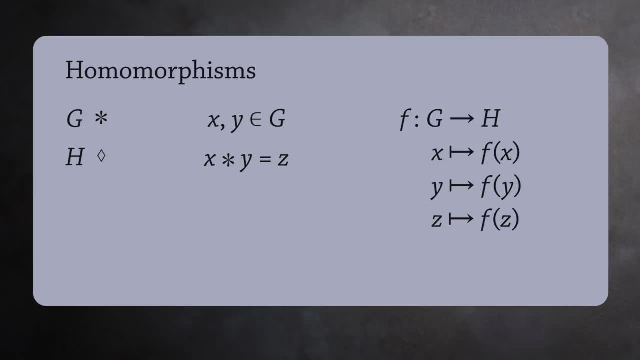 The whole point of a homomorphism is to find a structural similarity between two groups. So if x times y equals z in G, then we'd like f of x times f of y to be equal to f of z in the group H. But z equals x times y. Substituting this gives us f of x times f of y equals f of x times y. This is a definition of a homomorphism. 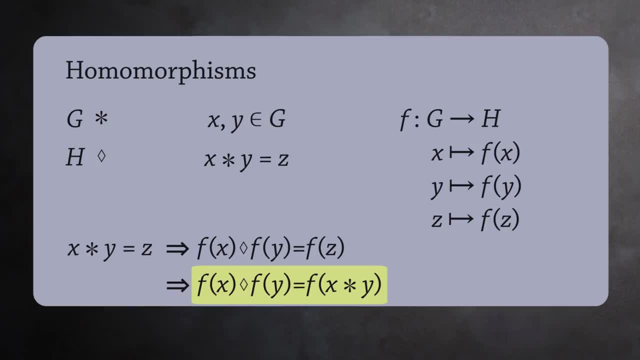 It's a simple definition, but it captures a big idea. A way to compare two groups. Let's see an example. 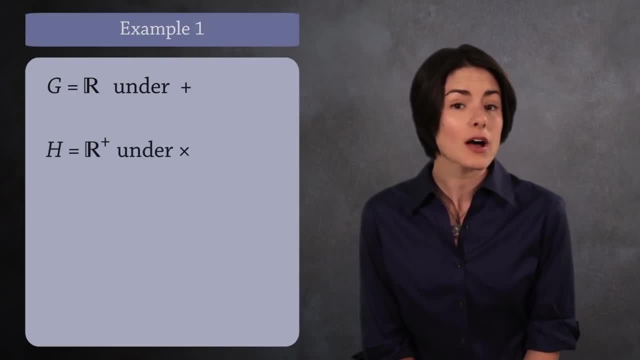 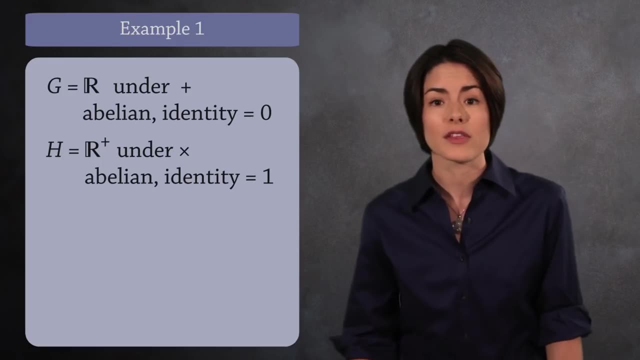 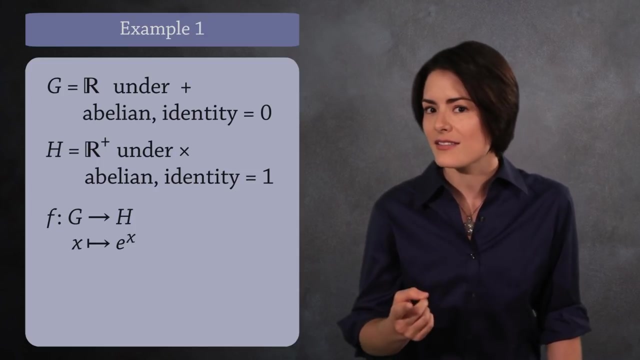 Let G be the group of real numbers under addition, and H be the positive real numbers under multiplication. G is an abelian group with identity element 0, and H is an abelian group with identity element 1. Here's a homomorphism. Define the function f that maps x to e to the x. 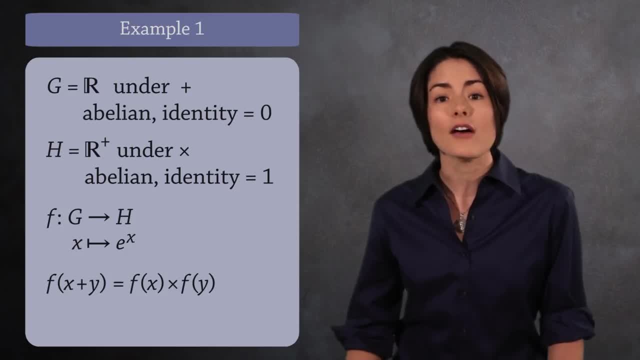 To make sure this is a homomorphism, we need to verify that f of x plus y equals f of x times f of y. Don't forget that the group operation for G is addition, while the group operation for H is addition. 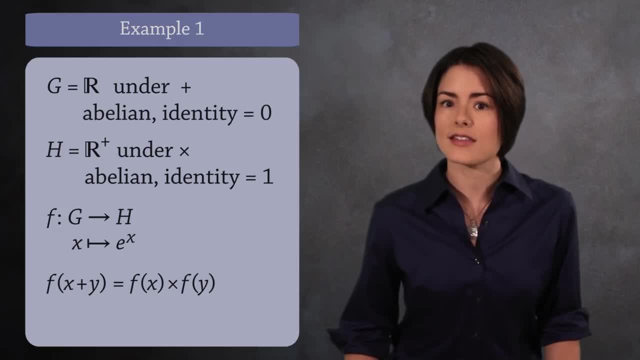 By the definition of f, this says that e to the x plus y equals e to the x times e to the y. And this is true. This is one of the rules of exponents. So f is a homomorphism.